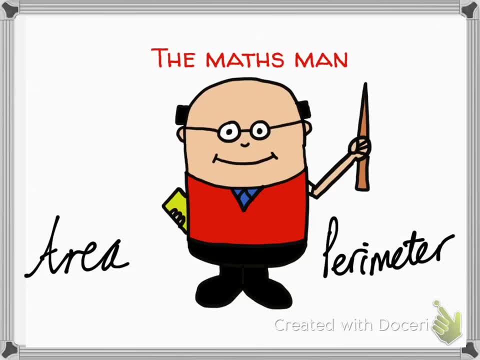 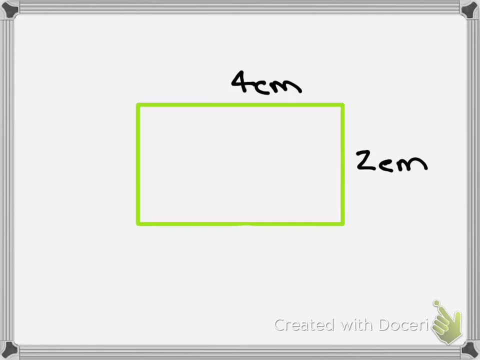 Hi guys, short video today. Today I'm going to show you the difference between area and perimeter, because a lot of people do get confused between the two, and I'm going to quickly show you how to work out both of them. So both of my examples are going to be with rectangles. So here we have a rectangle. I can see that this side here is 2cm, this side of the rectangle- and I can see that this side of the rectangle is 4cm. 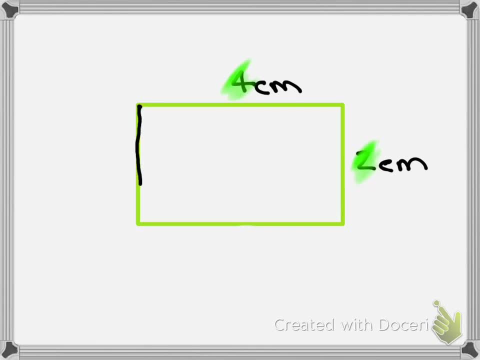 Now, when we work out the perimeter, we are working out the distance round the side. So I'm drawing round the perimeter now, So it's the outside of the shape. Now, to work out the perimeter, all you do is add all sides. 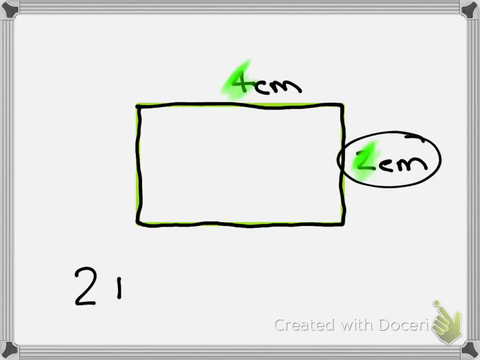 Now in my rectangle I have 2cm, add 4cm. this side must be 2cm as well, and then this side must be 4cm as well. So if I add all of those together, 2 add 2 makes 4, add 4 makes 8, add 4 again. 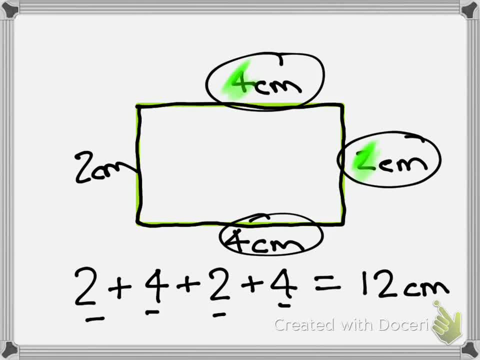 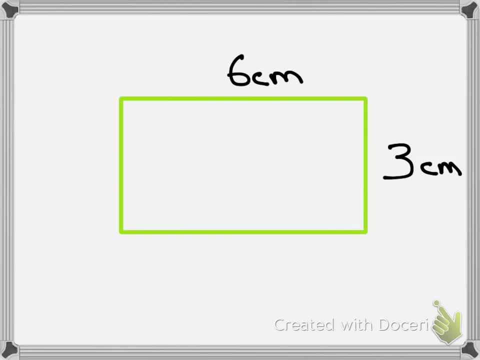 Again, it makes 12.. So the perimeter of this rectangle is 12.. Now the area. people do get confused with perimeter sometimes. Now the area is the bit in the middle. Okay, so it's not the outside, it's the bit in the middle. 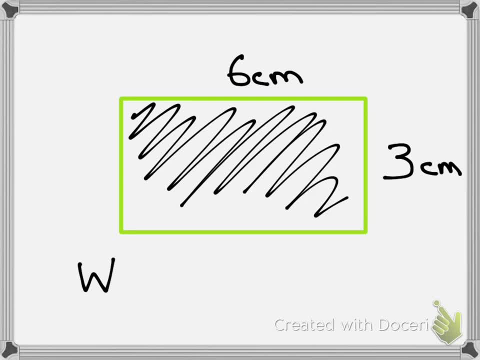 Now to work out the area, you times the width and the length together. Okay, The width on this occasion is 3cm and the length is 6cm. So if you add both of those two together, you get 18cm. 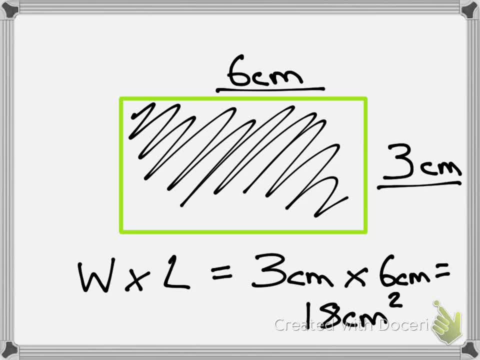 And because it's airy, we must put this little squared sign. so 18cm squared. Hope you found that video useful and if you did like it, please let me know with a thumbs up and I'll see you in the next video. Thumbs up down below.